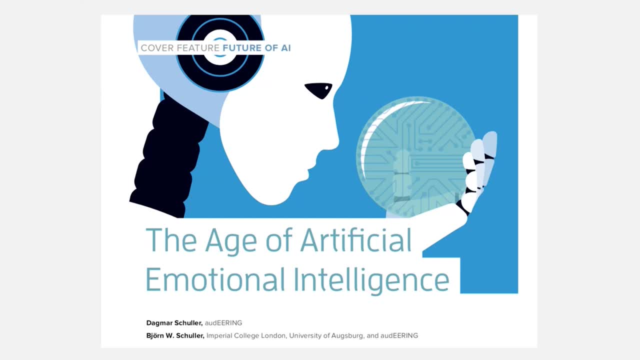 um, an interest in, um, what some people call artificial emotional intelligence. Um, and what does that mean? That that means a variety of things, right, Um, it's uh? um, it can mean simultaneously the simulation of human emotion. 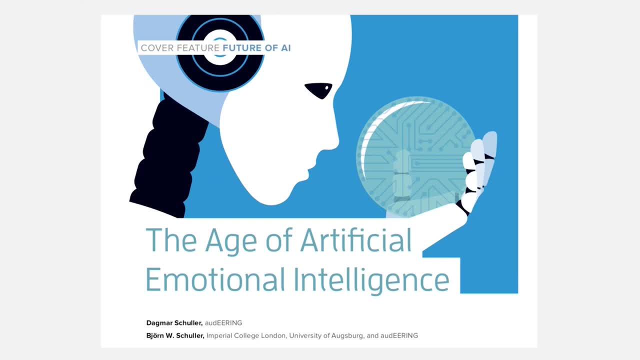 um by AI systems, or the collection and analysis of data about human emotions by AI systems And um the you know, there, there are various ways of doing this, um you know, and there are various, uh, various kind of. 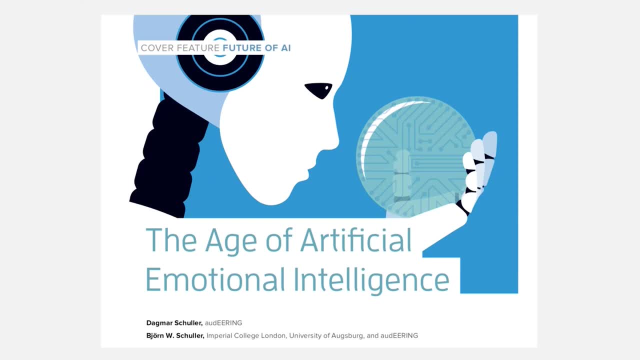 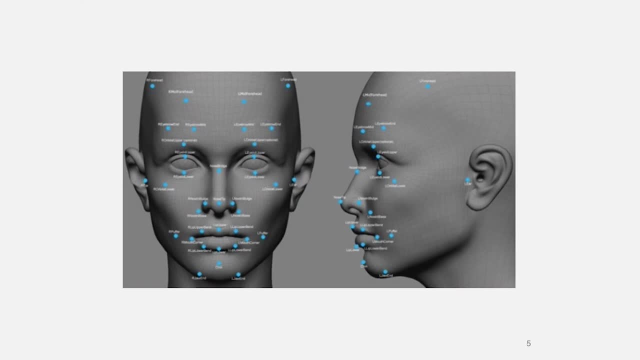 um modalities whereby uh digital technologies collect this information, The most um, of course, notable and and and probably highest profile being um emotion uh detection and analysis via facial, facial analysis, facial recognition identification systems. 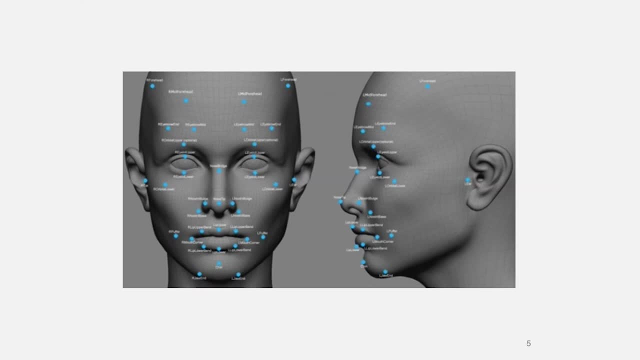 Um, but uh. so you know, this is, this is. this is of interest to me, in part because I'm currently writing a historical um monograph, a book on the history of how computer scientists have understood. uh. 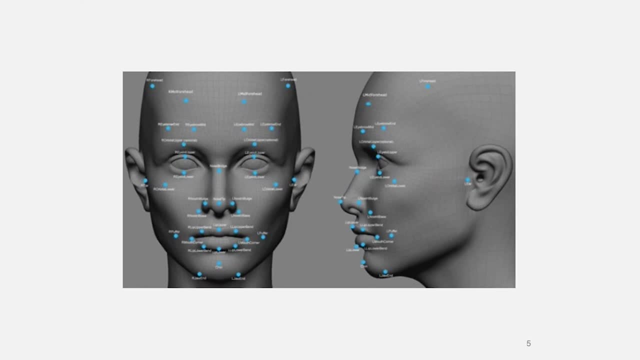 or misunderstood Human emotion. um, going back uh right actually to before, even the, the, um, the, the kind of invention of digital computers, uh, electronic computers And um, and so it's been fascinating to see. 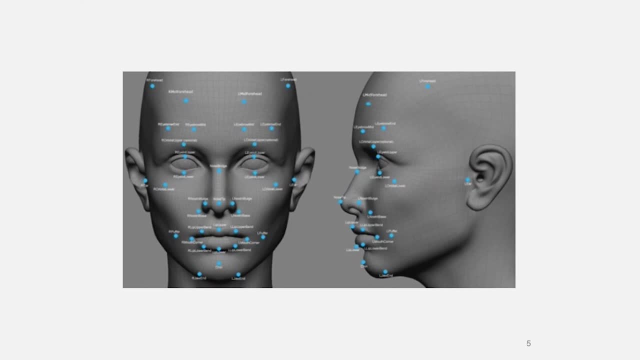 um, how that historical work connects with some of my kind of more contemporary work. um, and how many of the same conversations and, I guess, same sort of uh questions about what emotion is and how it might be understood via quantitative computational methods. 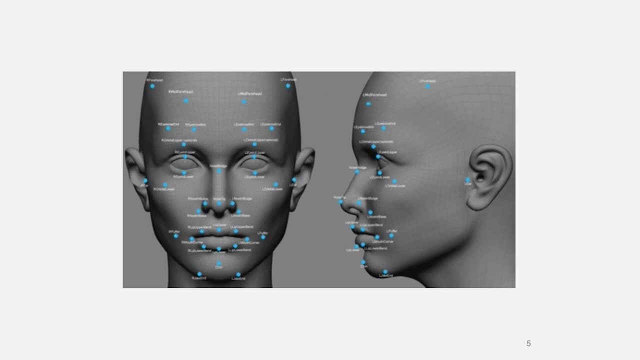 Um have really persisted over the past 60 or 70 years. Um, I'm not going to talk that much about that historical work um in the talk, but I'm happy to go into it in. uh the Q and a period. 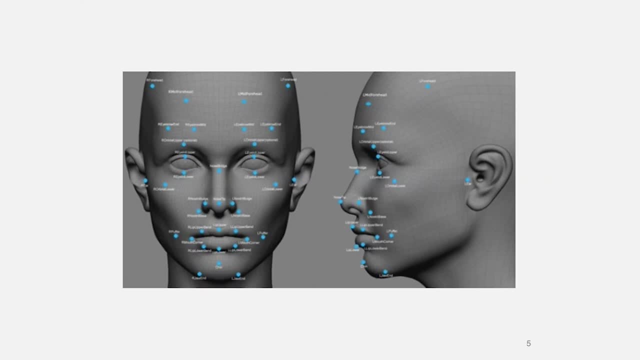 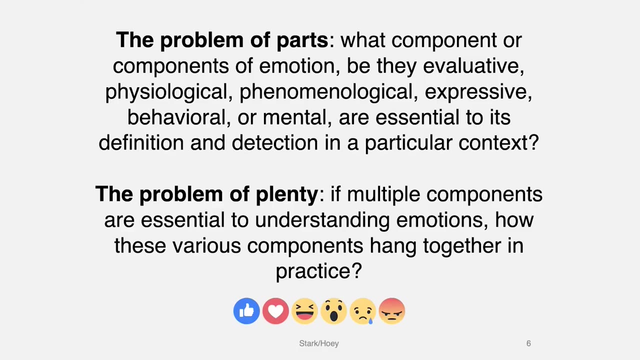 I, you know, as many of you probably know, being buried and completing a book manuscript you. it's really on your brain. So, uh, happy to chat about that as need be. So there are a couple of issues with emotion that. 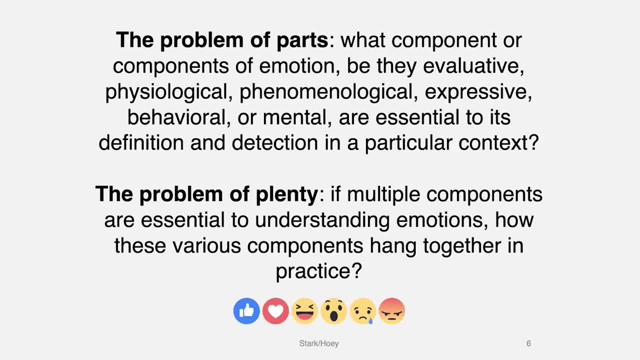 um, I want to flag before I sort of start digging into this work. and and why? why I you know what, what inspired it? One problem is, um, this question of the, um, oops, the question of the. 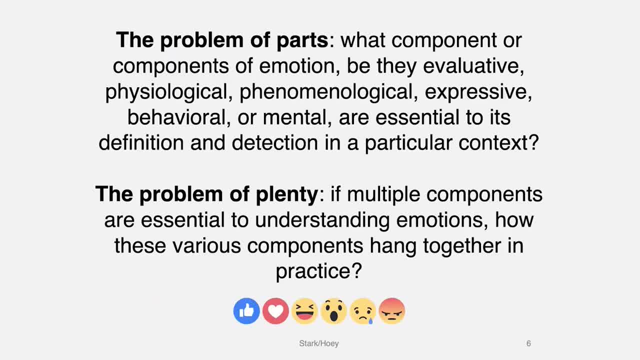 of what's the problem of parts, right Um? emotions are complicated, multifaceted, uh, multifaceted um phenomena, right Um? I think we can all understand from our subjective experience as human beings, right, That they involve both physiological responses. 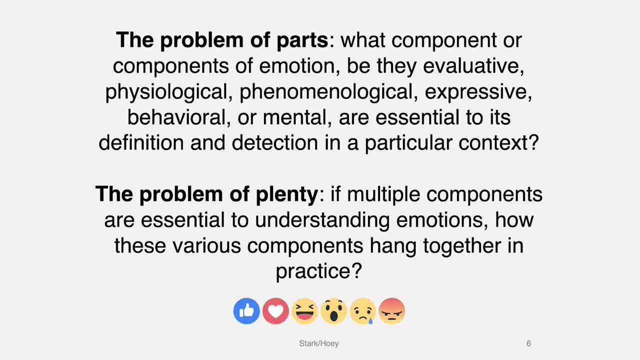 you know, getting flushed things, things in the body, um expressive behavioral responses, how we, how we react socially to emotions, um thoughts right, Our own awareness of, of feelings, uh, or lack of awareness um 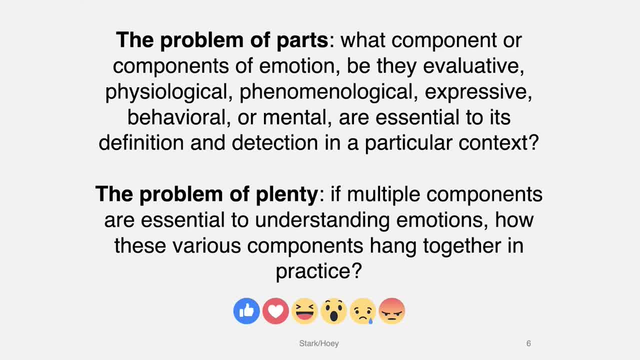 and, and you know, and various other facets, And so, so you know, the uh philosopher, Jesse Prince, who's a philosopher of emotion, talks about this as the problem of parts, right, What component or components of emotion? 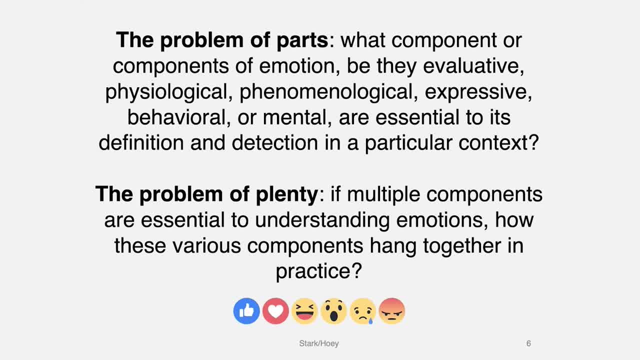 excuse me, are essential to its definition and detection in any particular context, because there are lots, of, lots of parts and you can't really capture them all all at once. And then the other kind of related point or problem that Prince brings up is this question, of course. 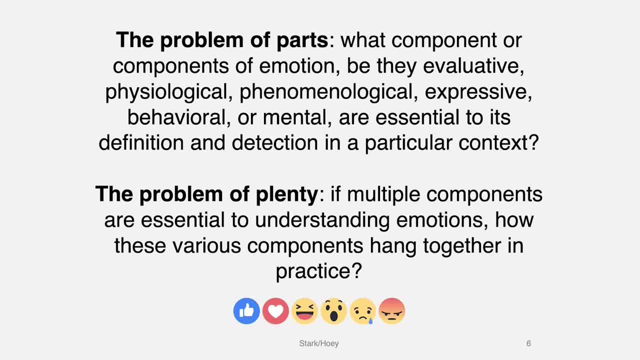 called the problem of plenty. right, If multiple components of emotion are- uh, you know, if most are essential for understanding it, how do these emotion components hang together in practice? How do they influence each other? And you know, and 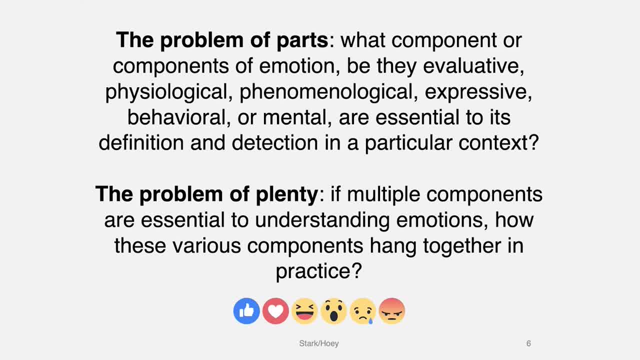 and, of course, for quantification purposes, for computation purposes, can you, you know, is one component of emotion a reliable proxy for others, And you'll see that the question of proxy um, proxy, um, uh for emotion is going to be really important in this talk. 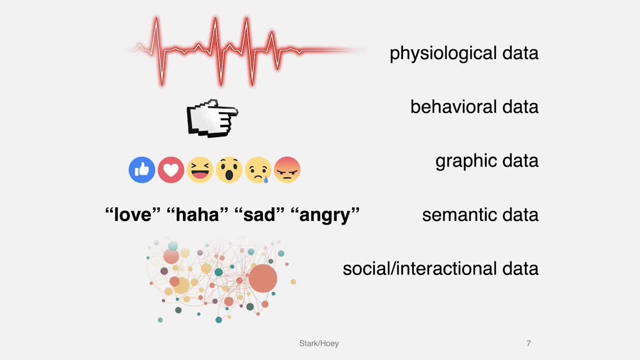 So, as all of you probably know, again I'm being being folks at a, at a major research lab. um, there are a variety of different proxy data forms that we can use to um to understand emotion, right, Um. 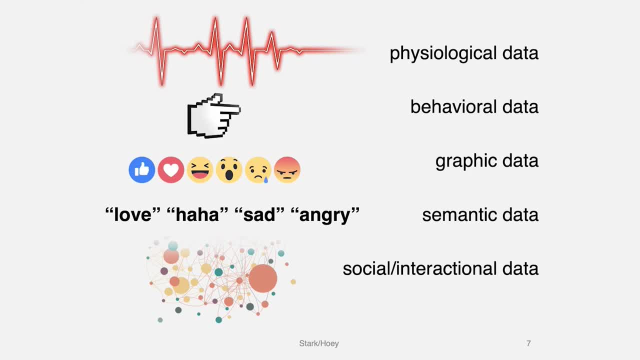 you know, there's physiological data um from heart rate, um facial expression, um skin conductivity et cetera. that also shades into the behavioral data right Um around around um response of the face or facial muscles. 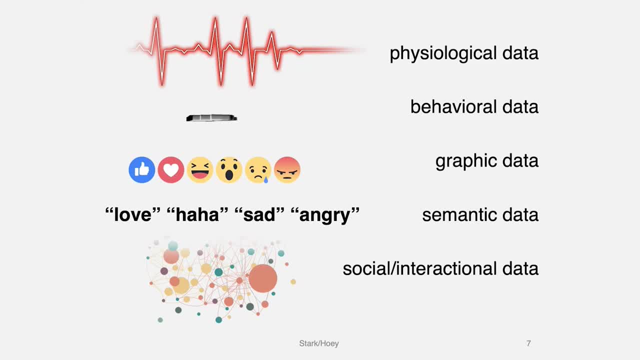 Um, there's kind of self reported graphic or semantic data, right? So this would be elements like um, the Facebook reaction icons or even kind of sentiment analysis with, with you know, dictionaries of emotion words. And then there are. 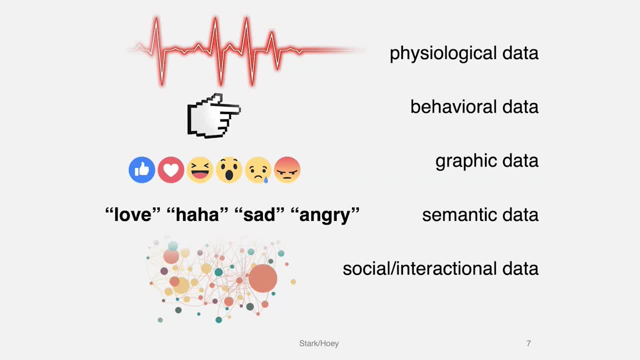 you know. then there's this whole universe of social and interactional data where you take these other proxies and try to kind of learn something from them based on um you know. you know, in social interactions between people over time, Um. 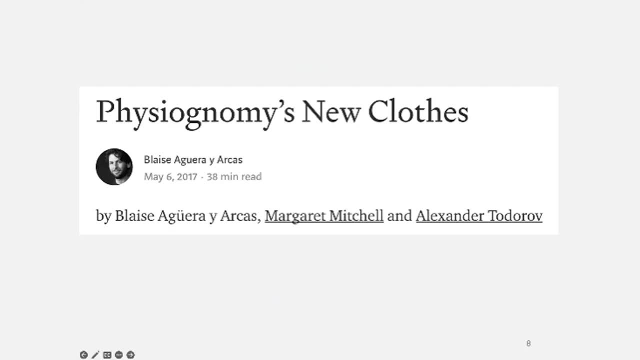 so, um, I'm actually going to skip that, this slide. I would just just it's here to say that, um, uh, you know, there there's a kind of broader question around emotion tracking, that that fits under into a kind of broader set of questions about what? 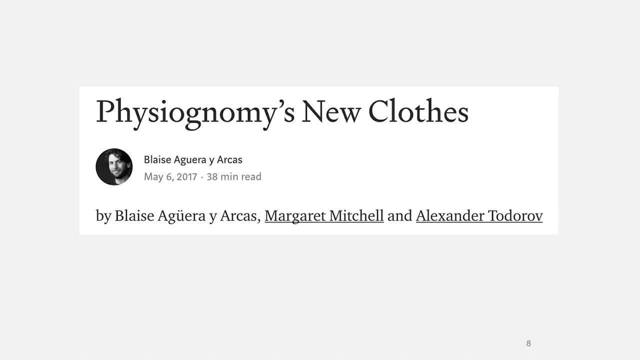 we can know about, um the interiority of individuals based on their exterior characteristics, right, So, um, in some ways, I think you could, you could lump, although in some ways, um, it's, it's, it's. 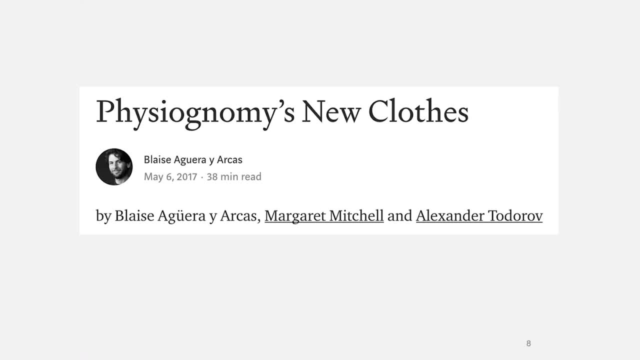 it's, it's, it's, it's, although in some ways not um. you could lump emotion tracking and analysis and contemporary uh computing into a kind of broader set of techniques that I and um another coauthor. 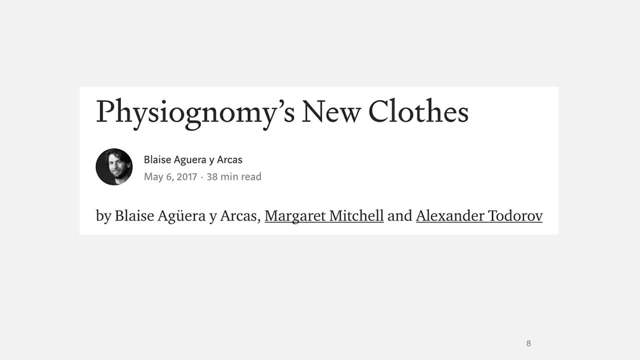 Jeven Hudson have talked about is physiognomic AI, Um, and, and so this is something else we could maybe talk about in questions, but there there's a, there's a. there's a real danger of replicating the mistakes of physiognomy. 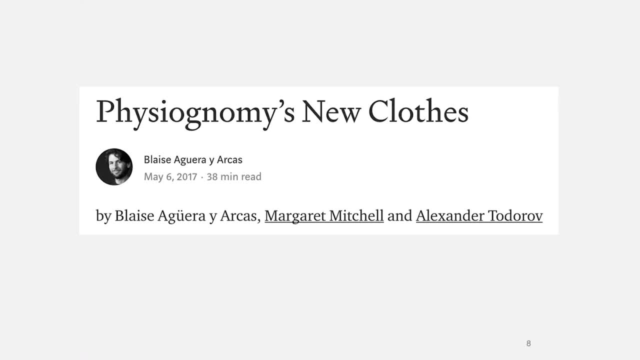 um, you know, replicating the idea that you can know certain things definitively about interior characteristics based on exterior, uh, characteristics, Um, you know, we don't, we really don't want to to to replicate those assumptions for lots of reasons in. 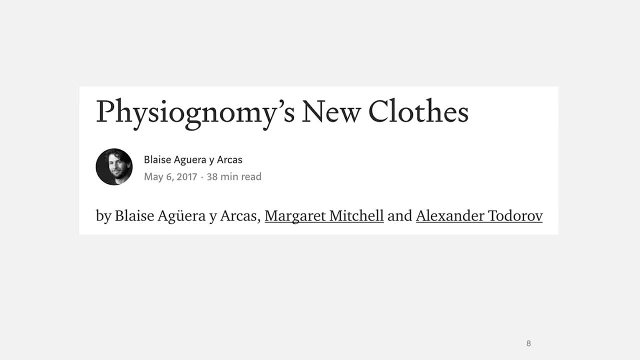 um in AI based analysis, And I'm I'm not the only person who said this- Um, some folks at Google wrote this really good piece- Physiognomy's New Clothes- um a few years ago. Um, and I. 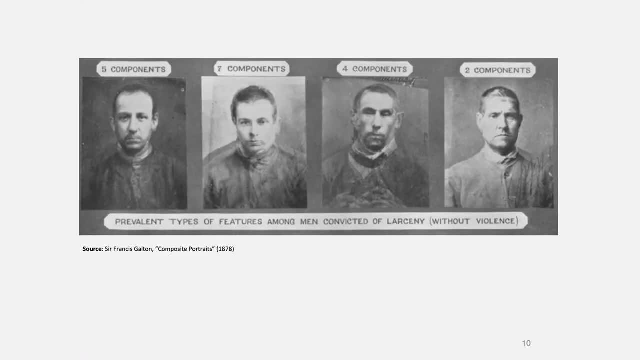 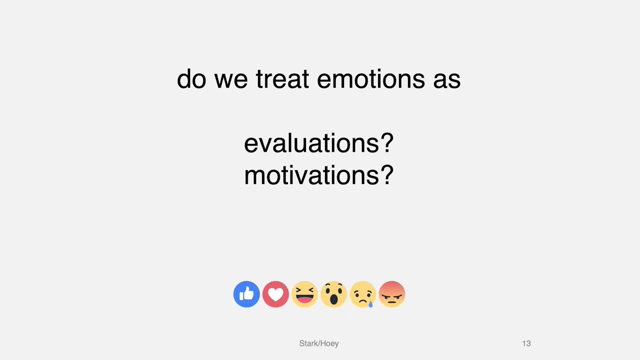 you know we were kind of in broad agreement. Uh, I'm just going to skip through those. So there's kind of a a, a central question, um, in the context of, you know, of emotion and emotion um, 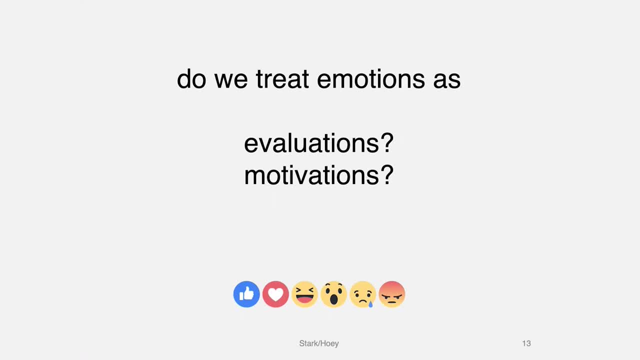 AI, um, whether or not we so. we have these different forms of proxy data right for what emotions are? Um and then. but then there are also a number of different kind of models for how we understand emotion, um. 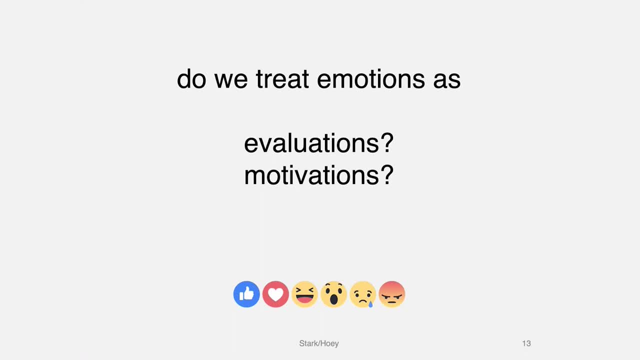 how we conceptualize what emotions are in the context of, of human um, you know, human mental life and and especially human um, I guess human theories of action and behavior and personality right, And I think you can sort of see. 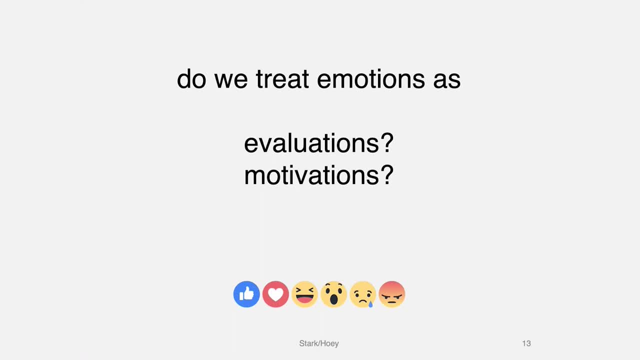 see them as as kind of um roughly- and this is very, you know, a very schematic about it- kind of kind of boiling down um roughly divided into two, two, um two groups, right Do. 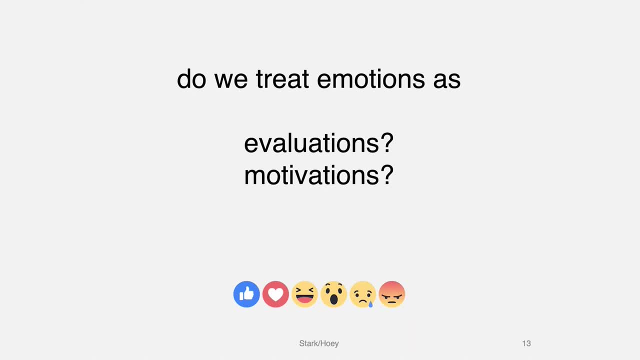 do we treat or understand emotion as you know- evaluative or motivational- primarily? right, Um so let's go into these in turn. right? Do we understand and do we treat human emotion as motivations, as motivational? Um so the? 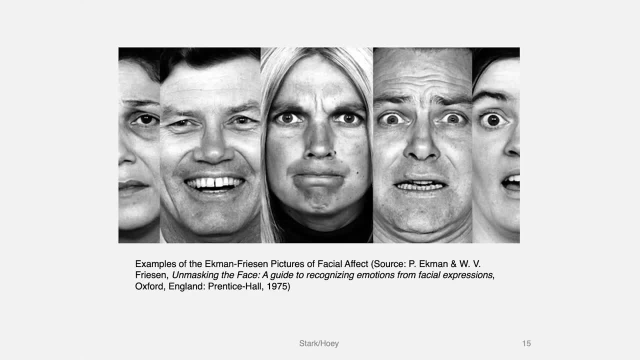 the kind of big champion for what we could call kind of motivation, motivational theories of, of emotion um in in effective science, and emotion science um is. is you know the work that I'm sure you're all. 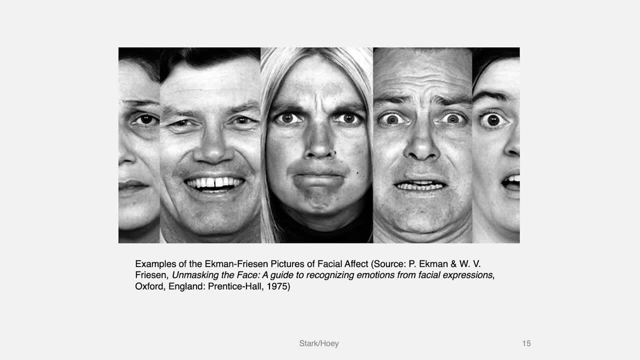 again all familiar with, of Paul Ekman right, The psychologist um, who in the 1970s really pioneered studies of emotion recognition in the face right He um did a variety of of studies both in the United States and then kind of cross-culturally and claimed that 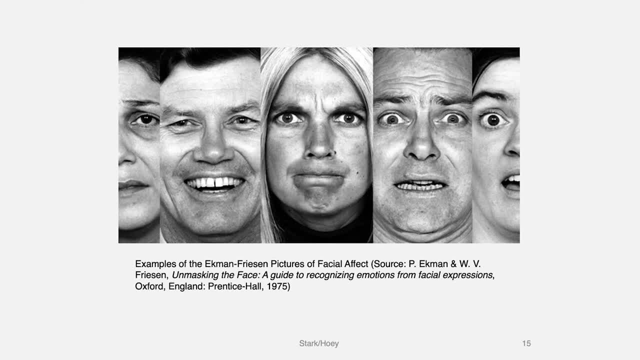 um, emotion could be understood as a a set of basically affect programs, right? So this is these are. these are. these are biological responses in the brain. They produce roughly similar responses, physiological responses across populations of the world, across all humans. 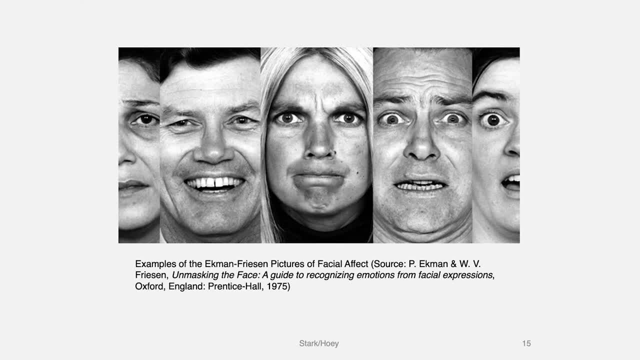 Um, and they can be narrowed down to five or six basic emotions, right And here, and here's a an image from the mid seventies, from one of Ekman's works, you know, displaying these probably quite familiar emotions. uh, 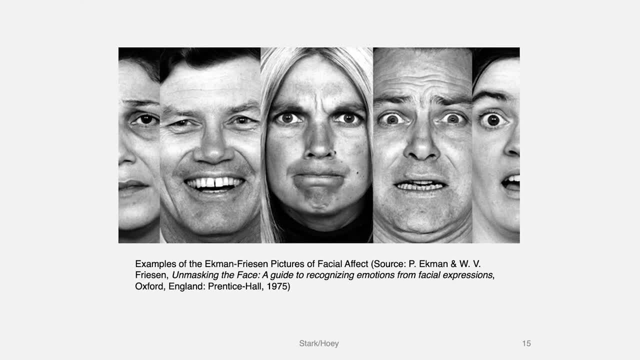 anger, happiness, uh sadness, uh disgust, et cetera. Um, it's important to note right That- and this is where some of the historical work that I'm doing does play into this, this question- that 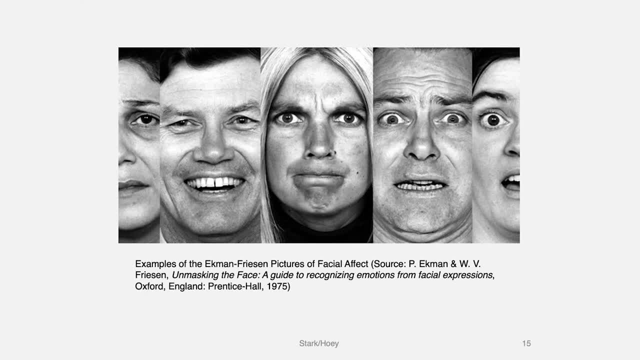 um uh Ekman was really heavily influenced and and and collaborated closely with um another psychologist, um uh Sylvan S Tompkins, who you know really um in his work in the 1950s and sixties really was. 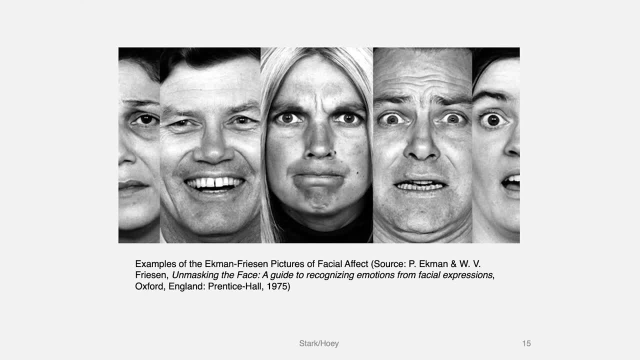 you know, basically invented this idea of of affect theory and affective programs as biological, physiological, um kind of motivating factors in human experience. Um right, And in some ways this was meant to push back against, um, the kind of 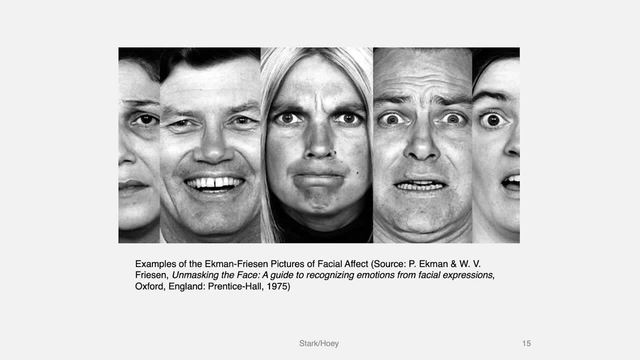 a kind of kind of radical behaviorism of of not ever thinking about the interiority of the brain at all. Right, Um, it was also a way of trying to kind of grapple in a in a kind of more scientific way with drive theory. 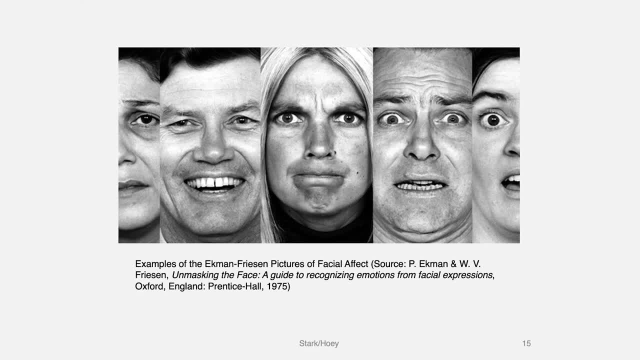 um from Freud and others, Um but uh, and, and finally it was. it was heavily influenced um, in ways that I think are are still a bit underappreciated by the cybernetic theory of Robert Wiener. 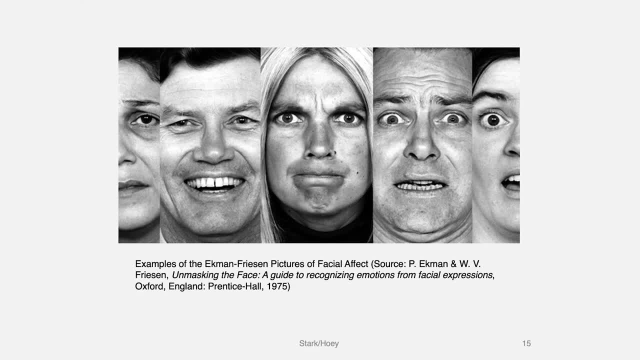 And and some of the ideas about uh physiological ideas about emotion that came into cybernetics via its relationship with physiology and um uh the work of somebody like uh Walter Cannon, if you know anything about the history of physiology. 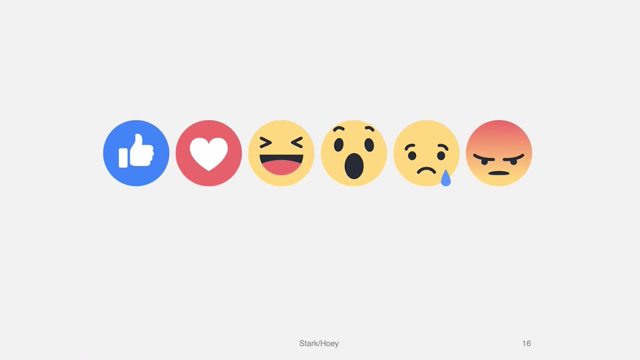 So um this motivational model of emotion, um which uh the historian Ruth Lathes calls um uh an anti-intentionalist, um model, um really pervades a lot of the digital artifacts that we see today online. 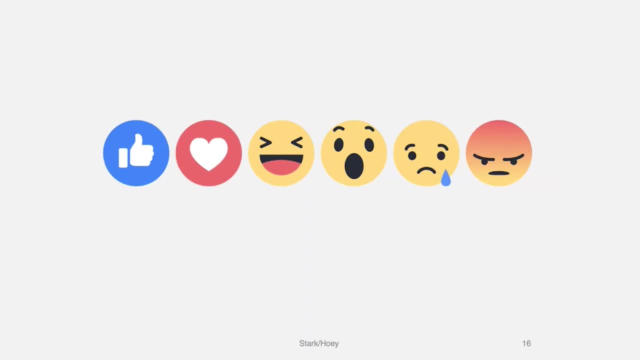 um that that have to do with emotion, Right Um it? uh, you know the Ekman group partially because the Ekman group has been extraordinarily um prolific in terms of its consulting and its influence in Silicon Valley. 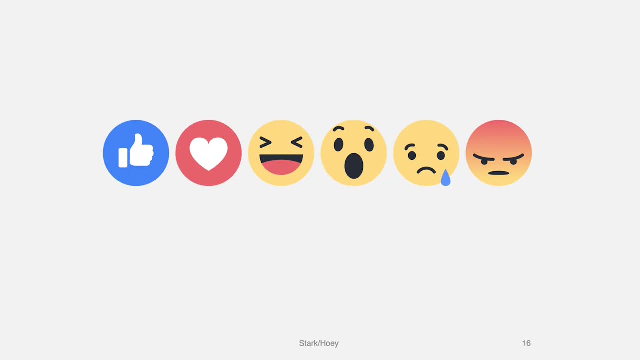 Um, right, Yeah, And, and the sort of basic emotion theory work um, pervades um artifacts like Facebook's reaction icons um, and and many other kinds of ideas about how emotion works, And you can see what the appeal of why. 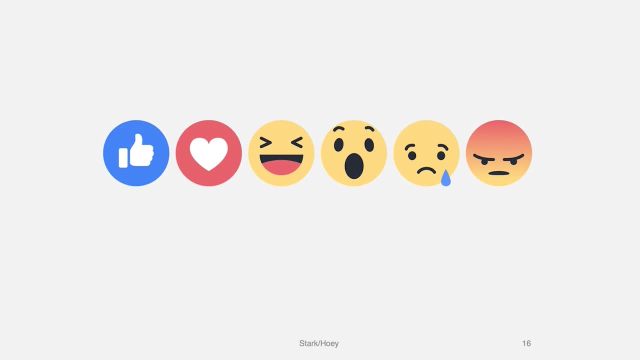 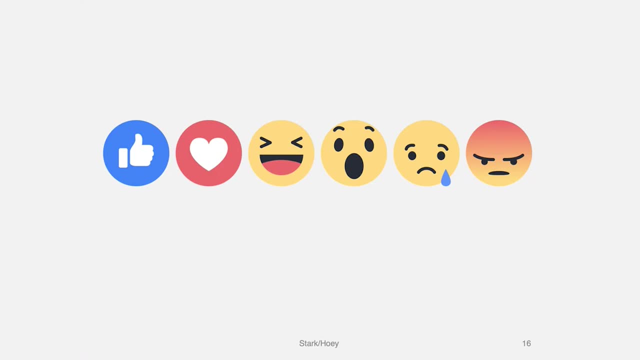 exists, especially in the context of computing, because it it suggests right, a kind of a kind of uniform, um ability to track and trace and analyze emotion, based on the assumption that that, whatever somebody's doing- smiling or frowning or whatever- 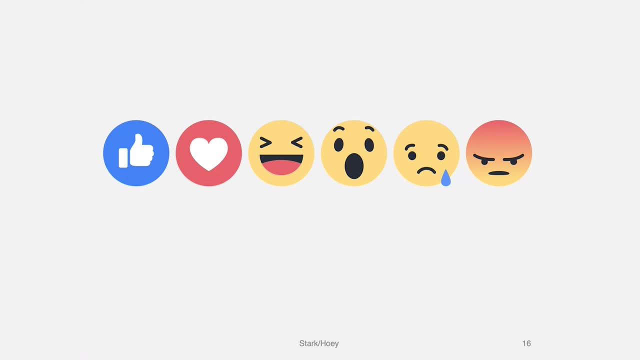 um, it's, it's giving some quote, unquote, true representation of how they're actually feeling, Um, and, and that you know, for for lots of reasons, um, and lots of applications in computer science, that that's obviously an appealing assumption to make. 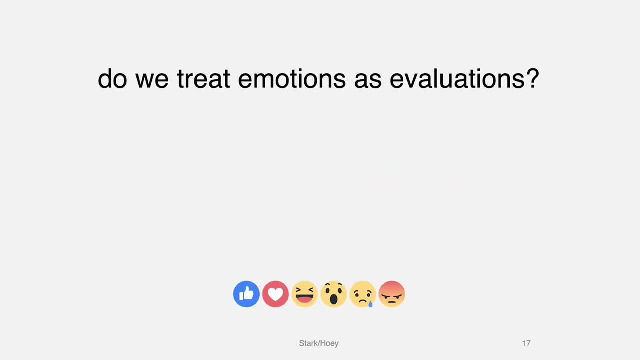 Okay, So, um then, the the kind of second, very broad set of of of kind of emotion theories or emotion ideas. um, is you know, this idea of treating emotions as evaluative? Um, and this, oops. 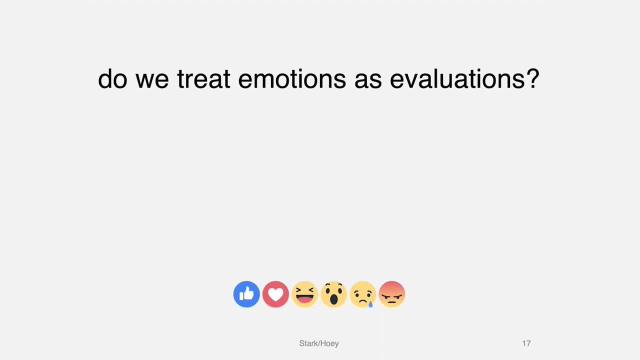 sorry this, um again. you know, out of a long history of emotion and emotion emotion work and you know psychologists talking about emotions are right. This, this, really this has a very cognitive science flavor to it. Um, 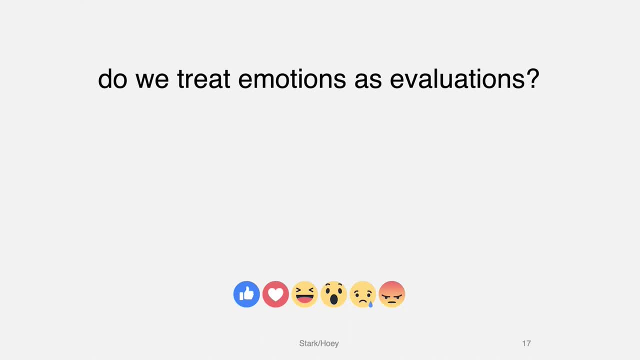 it. it really comes in in part with appraisal theory in the 1960s Um and and it and it suggests that emotions and emotional emotion response, um, are a part of a broader system of cognition. right That 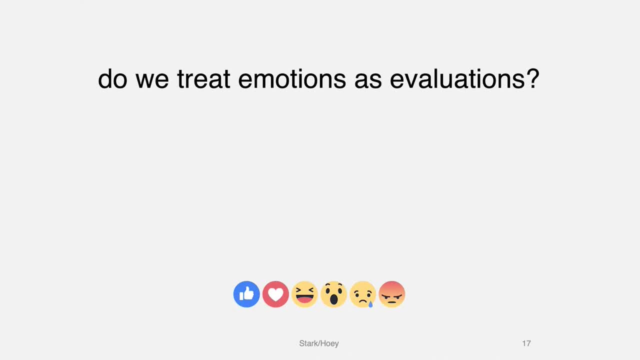 that, um that, uh, you know that that helps us judge the world and understand the world through emotional response. You can take this kind of kind of really far to the on the cognitive side, right, And so people. 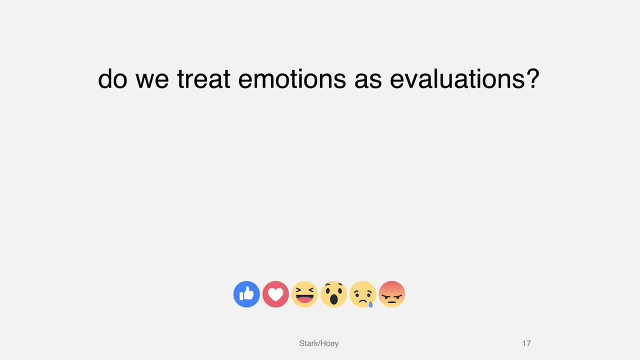 you know, talking about hot cognition and cold cognition as a way of, uh, as a way of talking about emotion without actually talking about emotion. Um, but there's, there's a sense, right That that, that this kind of cognitive science. 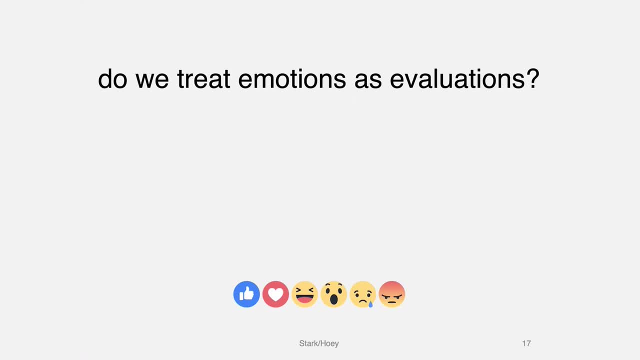 understanding of emotion, um, I think, in some models is a more balanced approach. right, That, that, that um, that we it assumes for one thing, that, um, that. you know, emotions are always something that we have to reflect on or should be reflecting on. 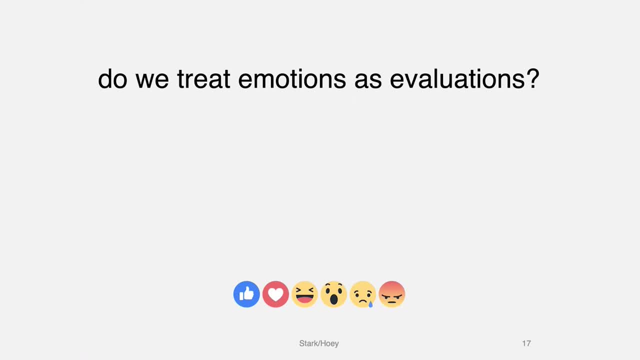 right. They're an element of um our experience with the world, And so you know, this is, this, is this is very much um a thing in social theory and some sociological work as well. So the 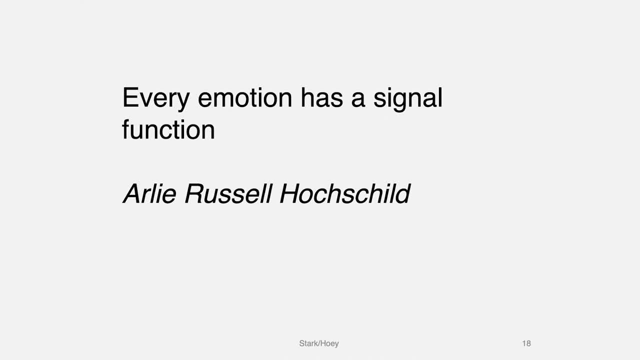 the very famous sociologist Arlie Russell. Russell Hogeshield, who um was one of the one of the first people to write about what we now talk about as emotional labor, right Had this idea that every emotion is a signal function. 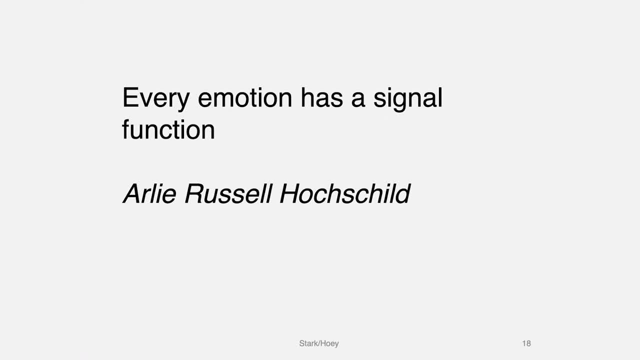 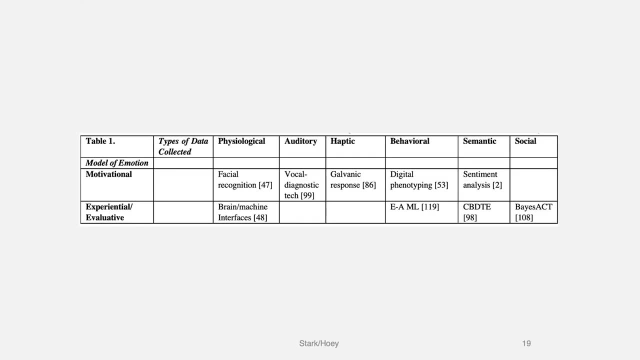 right That um that emotions are, are signals, you know, much like sense, impressions um about the world. So in the paper um that we published, in fact um Jesse and I, you know, first of all, 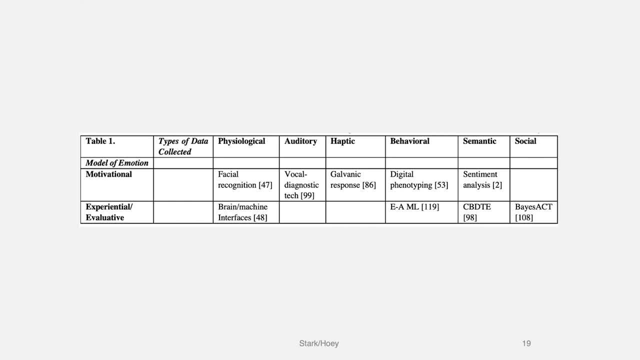 first of all kind of taxonomized this, this whole, this whole set of of um of types of physiological kind of proxy data collected about emotion, as well as models of emotion, right? So these these kind of two big ones. 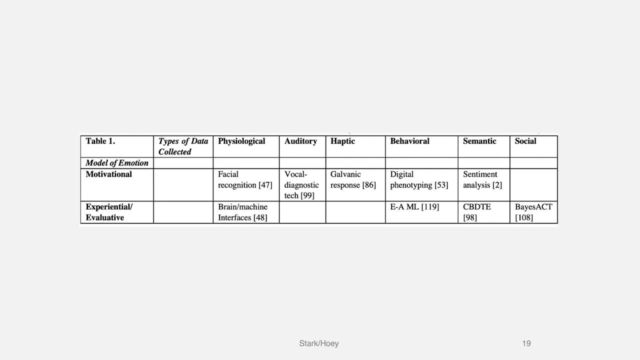 motivational and evaluative- sometimes you could call it experiential- And and one thing to really note is how, how much um the motivational model um persists in all sorts of different kinds of computational technologies. Um, you know. 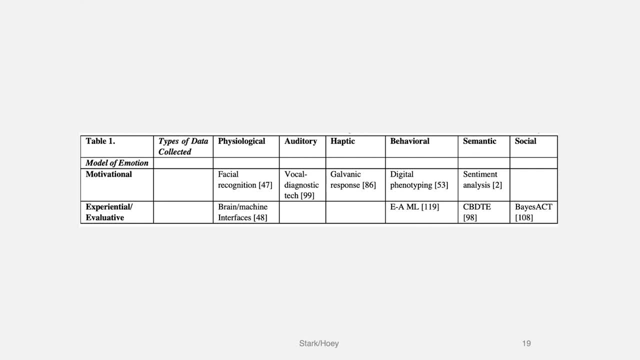 regardless of the kind of the kind of proxy data collected, right. So you see the motivational model in um areas like facial recognition in all sorts of, you know, emotion detection for speech, which is becoming a big kind of a big area. 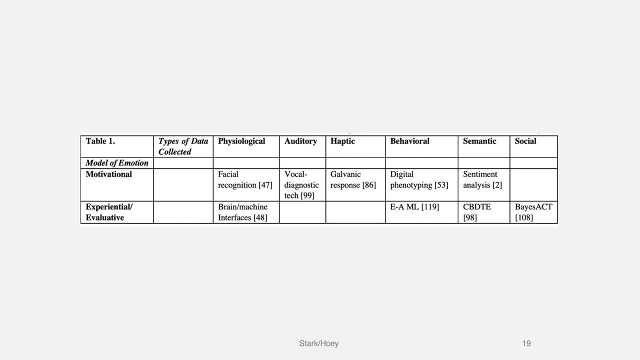 galvanic skin response, sentiment analysis, et cetera. Um, you know, models, digital models of emotion that are more evaluative are are a little bit less common. Um, there are some interesting uh attempts to structure. 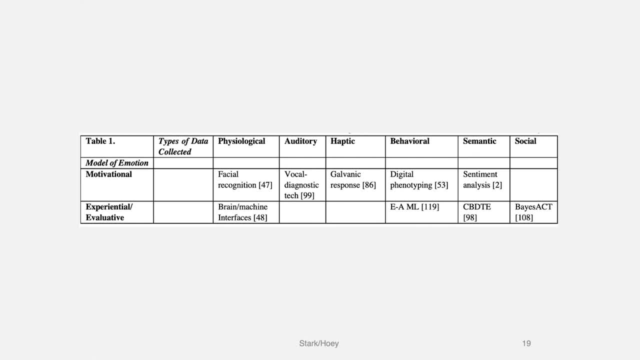 um uh, structure, AI systems, neural nets with a kind of emotion component, like a kind of emotion module, right, That is supposed to um try to mimic the role of hot cognition in, you know, human emotional response. 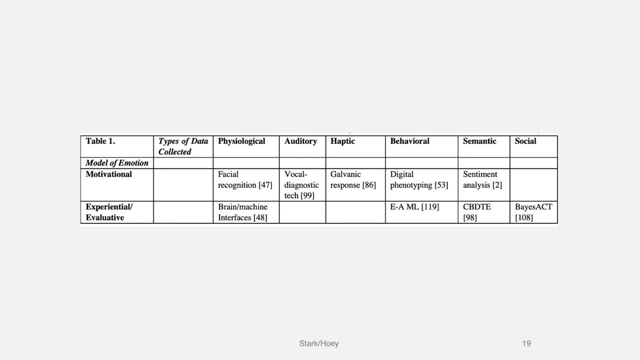 Um Jesse Huey, my colleague um is um is very interested in something called Bayes Act which, um looks, tries to incorporate kind of social norms around emotional response and emotional activity into the, you know, predictive. 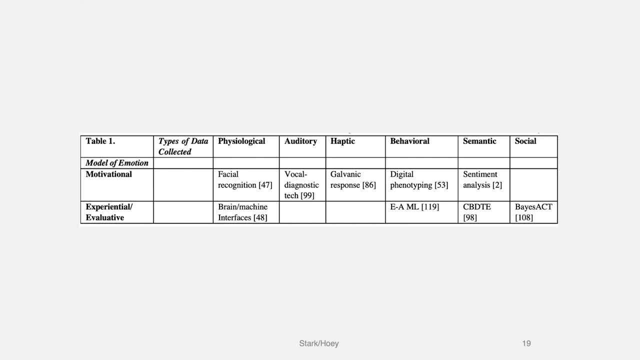 um, pr, predictive work with um with uh, with voice agents, for instance. But in general, this motivational model is much more, much more powerful and much more present, And so I think one of the you know, 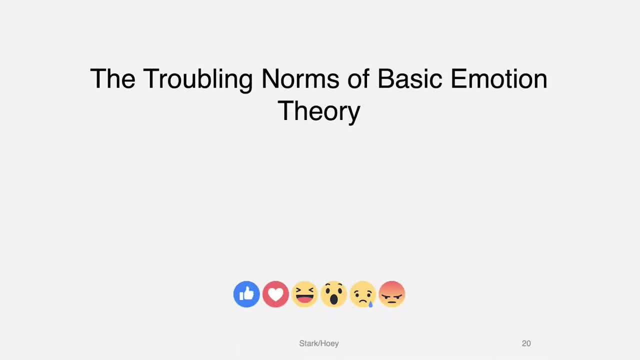 in the, in the second part of this, the paper, um, we, uh, you know, become really interested in and talk a lot about: um, these questions about the kind of, the kind of troubling norms, what we call the troubling norms of basic emotion theory. 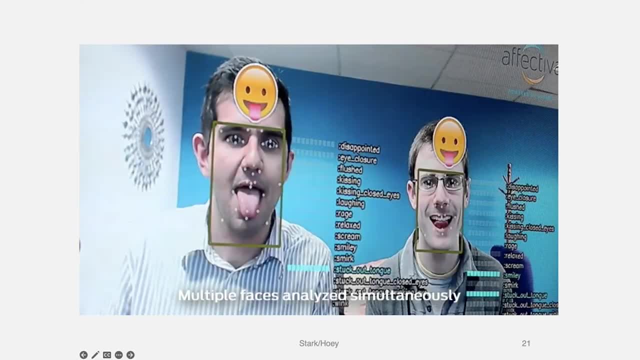 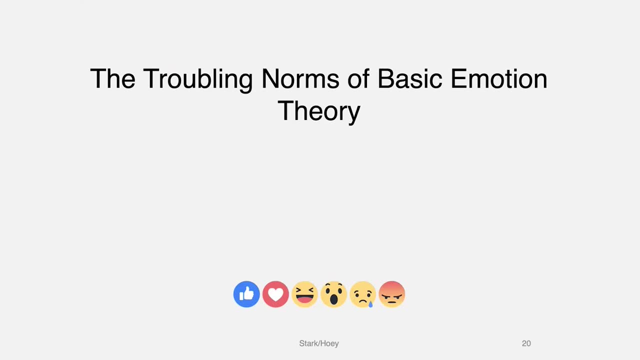 Um, and and sort of. fundamentally, why basic emotion theory? oops, why basic emotion theory as a kind of a kind of assumed ethics and assumed um, uh, you know, assumed state of of human, um, autonomy, your human. 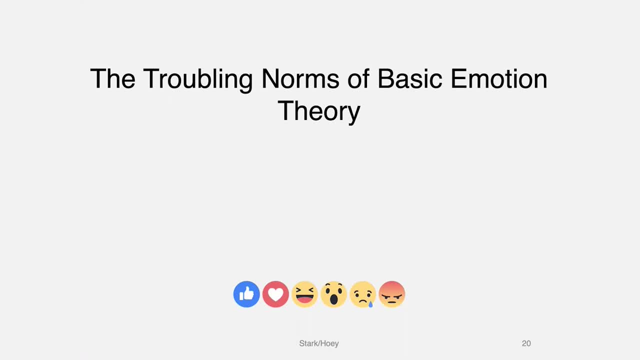 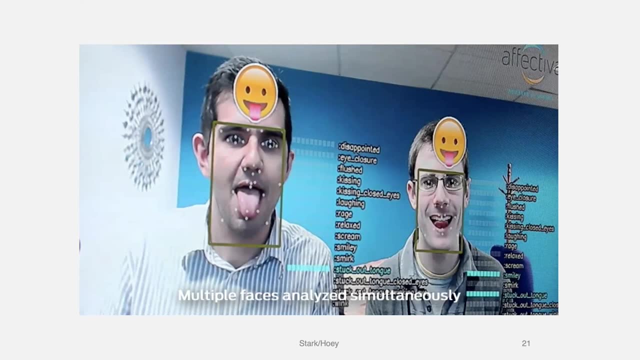 uh, activity, um is kind of a problem, right. So you know, as I- just you know- did this kind of motivational theory of emotion as, again, as I say, it's very, it's very common and very popular. 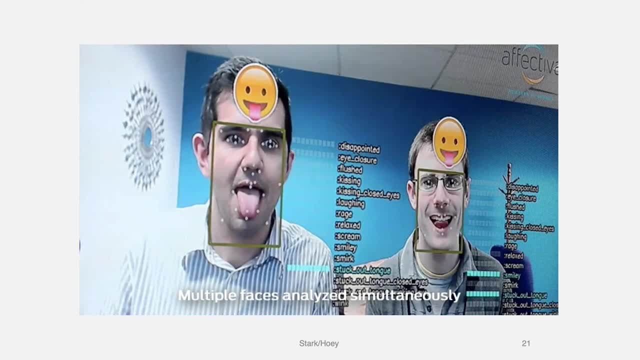 right. So it it persists across um a variety of different, um kind of online online marketing or online- um uh, firms that that use these technologies, maybe the most famous being Affectiva right, Which came out of the MIT Media Lab about 10 years ago and has now been purchased by Smart Eyes. 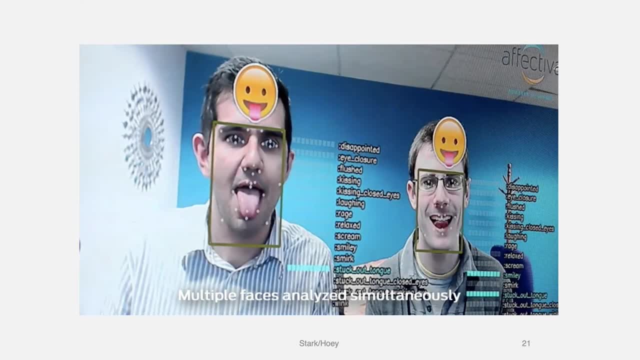 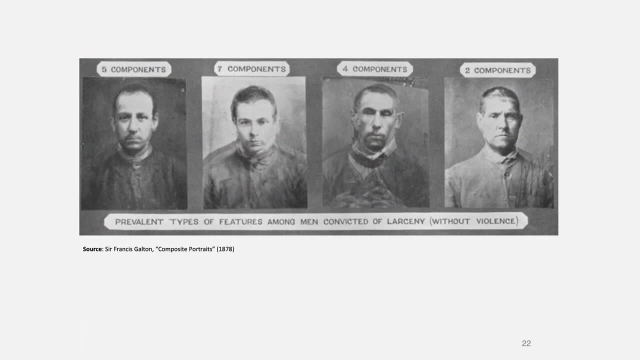 which is a big car, um, emotion tracking company, Um, and I think one of the things that that concerns us or troubles us about the, the kind of the kind of the norms of basic emotion theory, is this connection to this broader discussion about physiognomy and 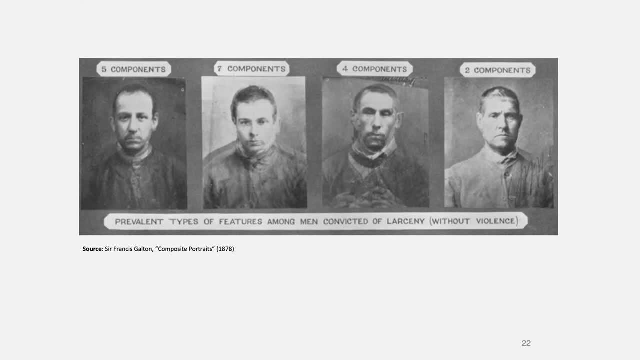 and its assumptions about the interiority versus exteriority of humans. Um. this is an image from um the work of a very noted 19th century statistician and and um physiognomist, um Sir Francis Galton. 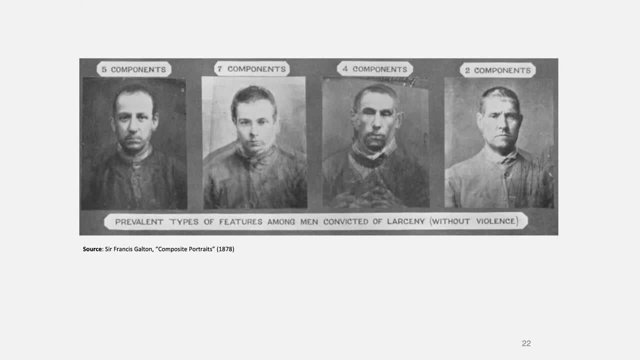 right, And you know. so, just just to give you context, what. what what's happening here is Galton is trying to infer criminality, um, through exterior facial facial features. right, He's trying to. he's overlaying portraits of people who have been convicted for crimes and trying to see if 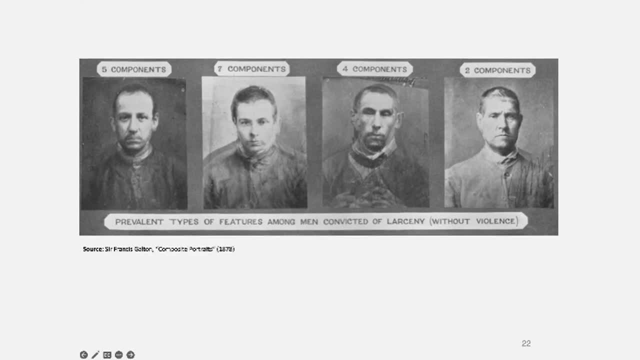 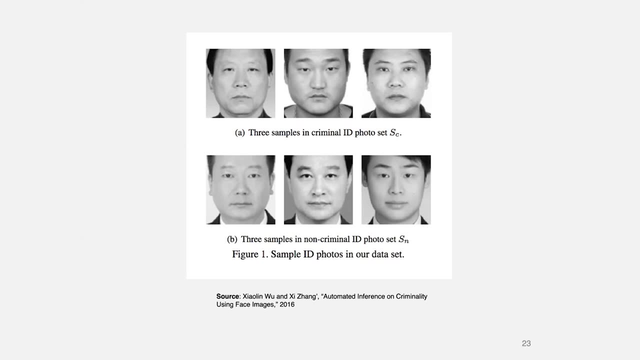 you know if their noses look all the same to kind of figure out this kind of criminal nose. Um, and you know, and we've seen sort of similar, you know similar kind of controversies around similar, directly sort of physiognomic papers involving crime and criminality. 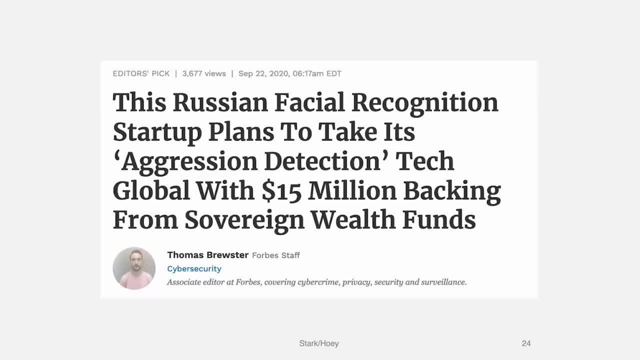 This is a famous one from a few years ago, But I think, you know, we we also have to think about the these, these, these questions about, about interiority and exteriority, um, in the context of emotion. 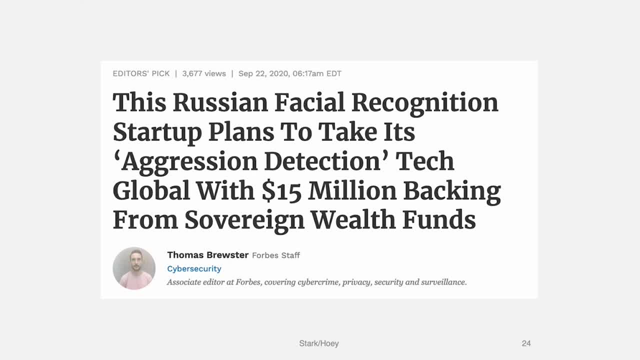 right, Um, this is a somewhat dated example, but um, you know, um, there are lots of, lots of kind of of, kind of of startups and and and other um projects that claim to do things like. 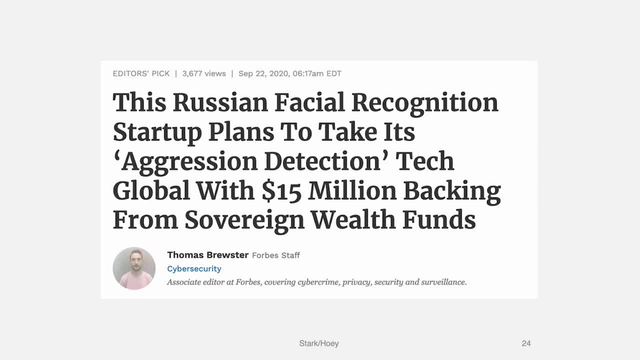 you know, detect aggression, detect guilt, uh, or detect other other kind of, you know, potentially problematic negative emotions using facial recognition technology and using other technologies. Um and and again. right, this really relies on understanding emotion as a motivational force in human behavior. 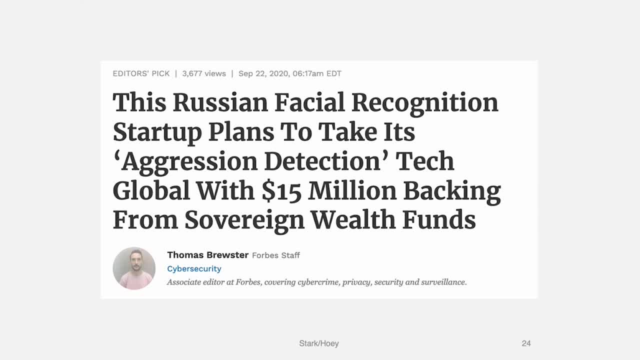 right That you can't hide your guilt and your guilt will be displayed on your face. Um, those are the kind of the kind of conceptual assumptions underneath these technologies. Now, there are a bunch of issues with this. What one of which. 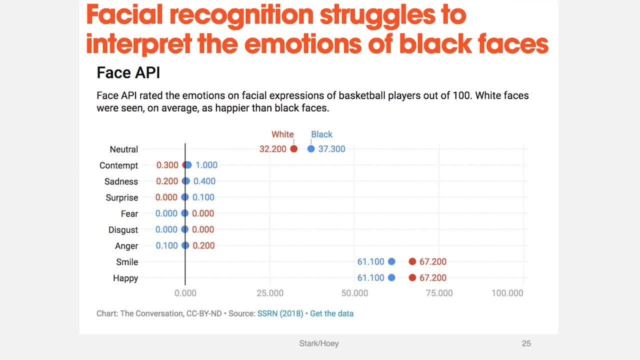 you know, ties into a lot of the recent work in the kind of fairness and bias um literature and and responsible AI, which is that, um like many other facial recognition systems, um, these technologies are not very good at interpreting the emotions of certain groups. 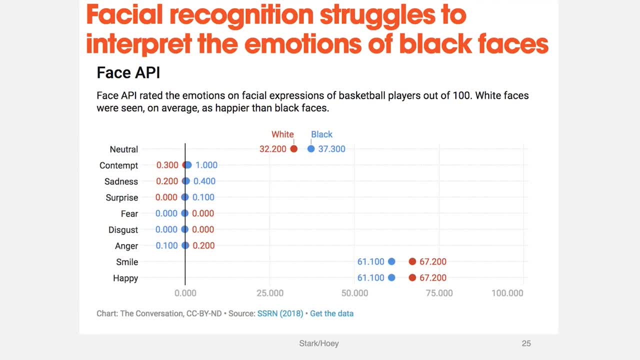 particularly um black faces right? Um. this has to do in part because of training data, um it has to also to do with facial recognition. It would also has to do um with um the fact that a lot of skin connectivity 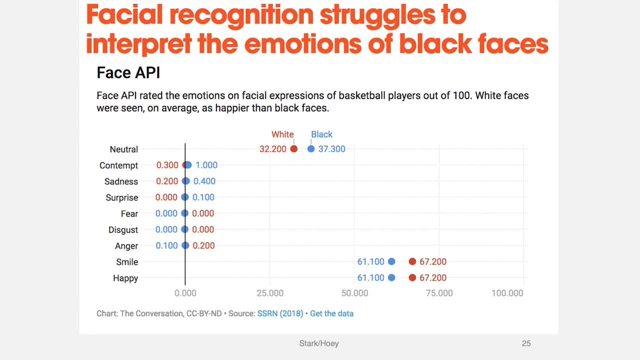 um, technologies are not calibrated for darker skin tone. Um, and so this, this, this um. this work is from, uh, Lauren Rue at the University of Maryland. Um, she did a really great study where she shows how. 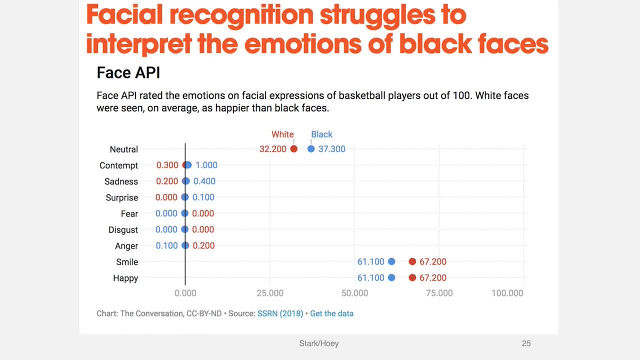 um how much worse um the commercial face APIs are at detecting um happy um smiling black male face than happy smiling um white male face. She did this on on shots of um basketball players. 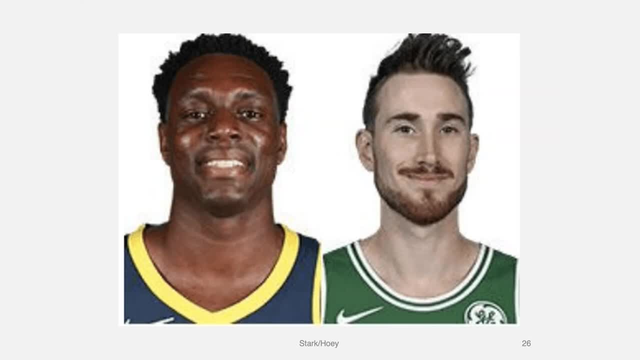 um, you know a kind of, a kind of controlled data set that you know, so you know everybody in these data sets is is, you know, an? a, a male athlete smiling. Um, and these systems are much less likely to identify the face. 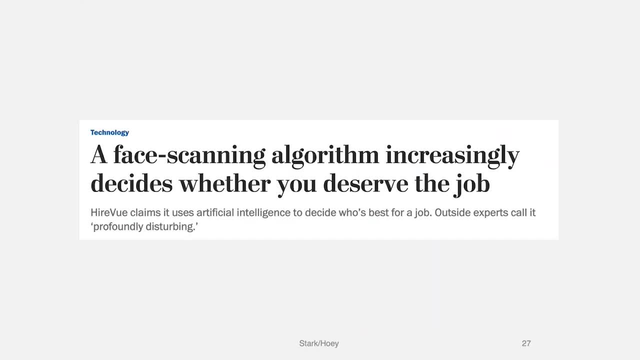 um of the black athlete is smiling than the face of the white athlete. So right, I mean, this is this, is this is not simply an academic problem? Um, uh, given how, how common a lot of these things are becoming in. 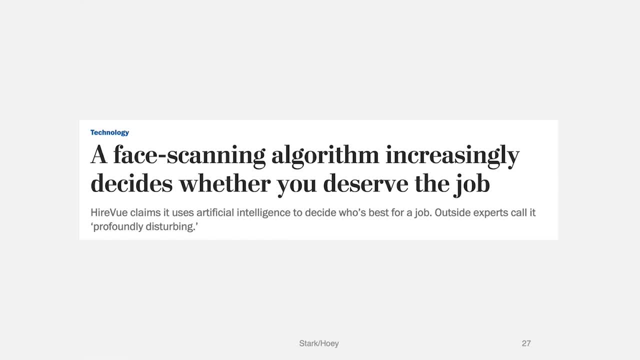 uh, areas like hiring, um, border security, um, and, and many others, And we could- you know, there's a whole list- um you know, the more that these systems become become used to adjudicate um. 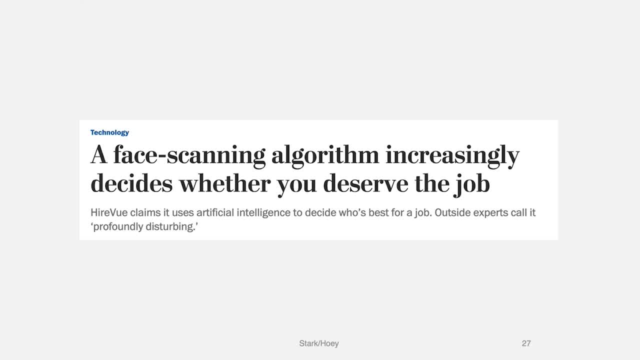 and judge your interior state via emotional expression, the more of these problems are going to crop up. Um, and these problems are both these kind of technical problems around, um, whether the system is, uh, treating everybody the same way, but also more critically. 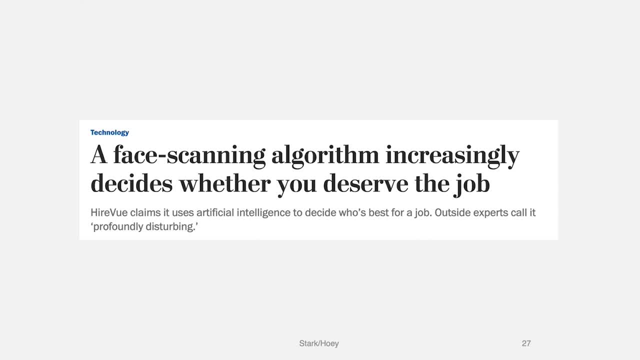 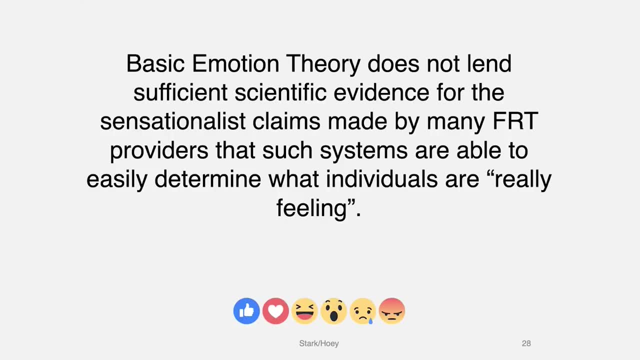 these conceptual problems right, Assuming the motivational nature of emotion, when in fact that motivational nature of emotion is really heavily contested. right, Because here's the thing right: Basic emotion theory does not really lend sufficient scientific evidence to um a lot of the claims made by kind of facial recognition providers that 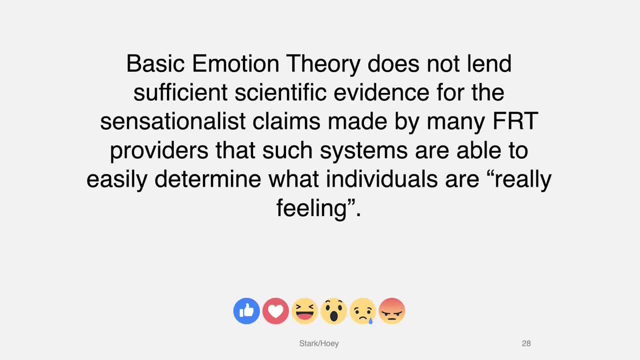 that these systems can really easily determine what people are are really feeling. um right The the kind of critiques of basic emotion theory um we've been seeing concerns about it um go back into the 1980s. 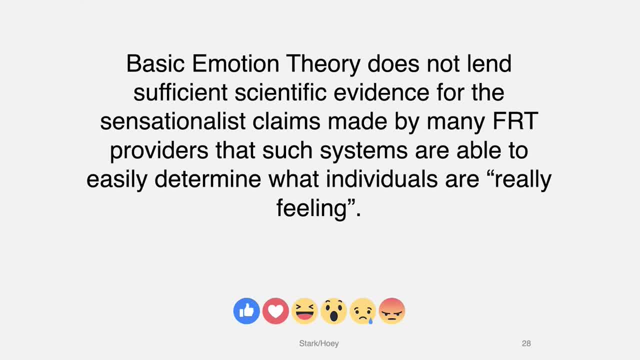 1990s um with folks like um James Russell, um more recently, um, uh, Lisa Feldman Barrett at Northeastern has been a a kind of major proponent of of you know different. 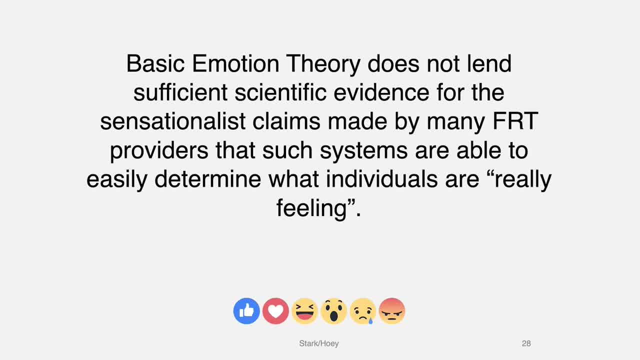 you know different, more complex theories of how physiological affect shapes human emotional response, right, But but the idea, and and she did a big meta review a couple of years ago that showed that really these, you know this idea that there's a kind of 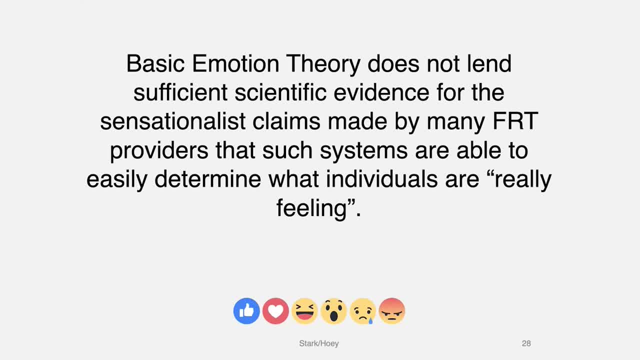 a kind of a kind of reliable correspondence between um emotive expression on the face and um, and you know, subjective understanding or feeling. you know it really just doesn't hold up. So the you know the. 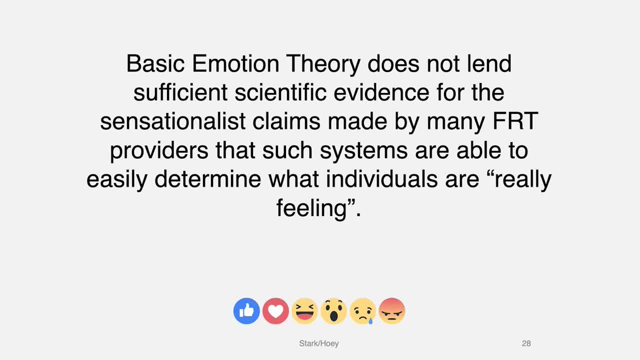 the discourse amongst researchers, I think, is significantly more sophisticated and more um more nuanced. right Then the conversation that's happening often in the commercial realm, right The way that, the way that you know these technologies are getting spun by marketers. 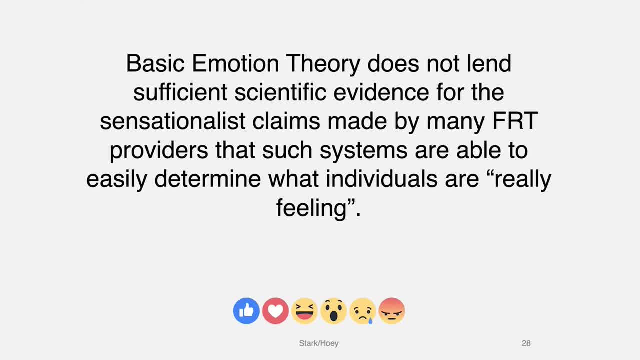 Um, and some of those claims are, are really very sensationalist. Um, uh, you know, but again you know, these, these systems are, are, are, are kind of kind of becoming, uh, highly ubiquitous. 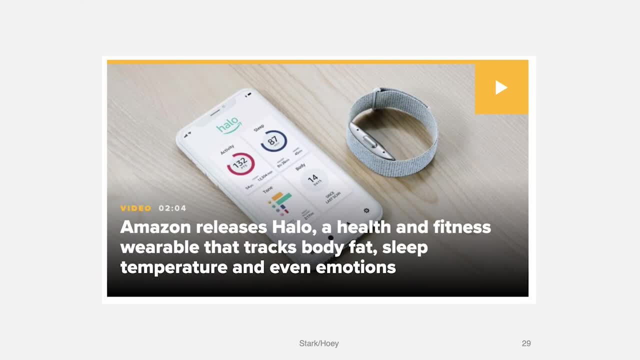 right, Um and um. so another concern that we have in the paper is really um, really how, the, the, the kind of preponderance of, of this motivational model of emotion, how, how, you know how? 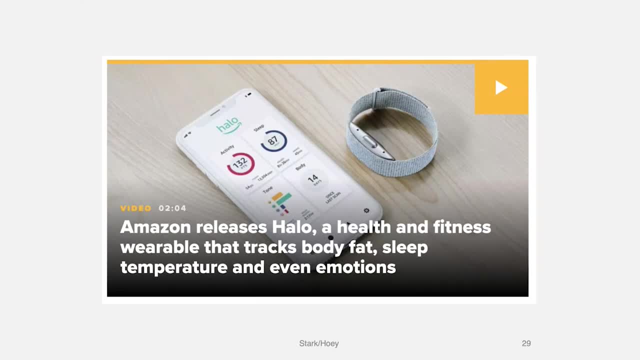 how it, how, what? by circulating in the world. what does this belief that that emotions are motivational, what? what effects does that have? And, and, and, and, and, and and um, the science is. 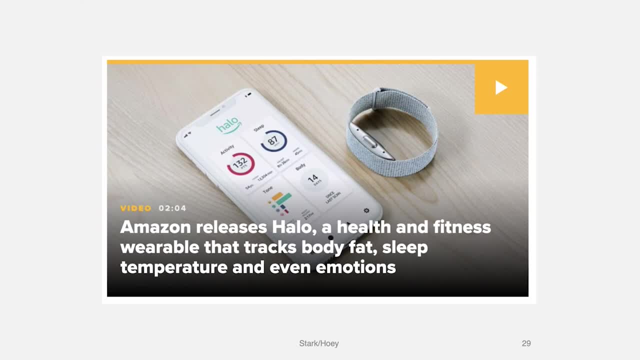 is is unclear. The science is, in fact, not very good, but, um you know, people are very good at acting as if, um you know, are shaping their behavior around their beliefs, And so, um right, we have a big concern that. 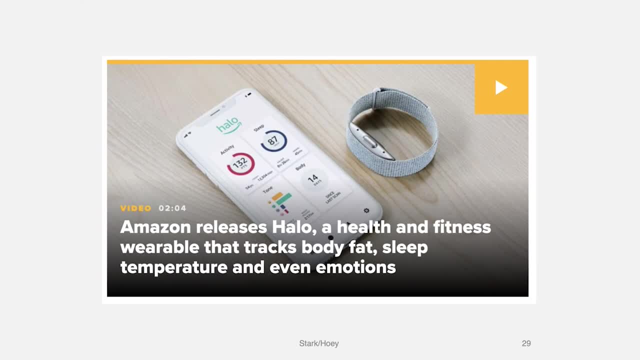 um, that people will sort of, will sort of begin to believe in these external signs or signals of emotion, um, and and kind of understand their emotions as being motivational, And so, um, I, I think it's, I think it's. 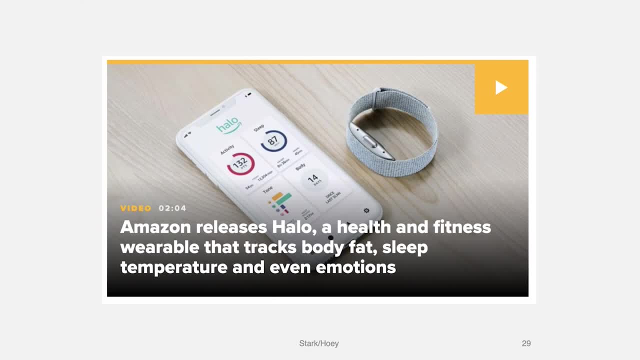 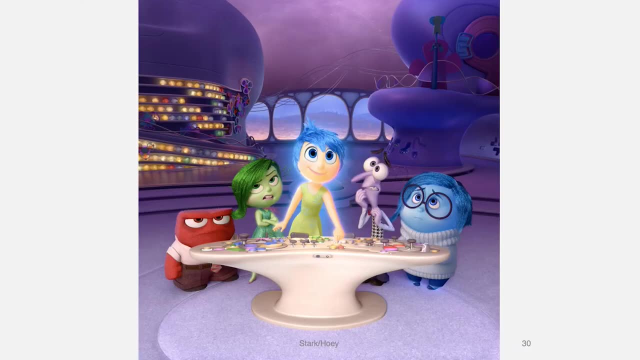 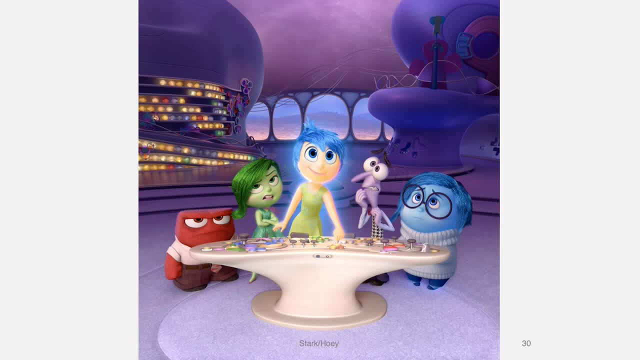 And you can see this, you know, not just in consumer tech but in um. you know cultural products like, notably, um, the Disney Pixar film Inside Out from a few years ago, which um was also based on Ackman's basic emotion theory and has all sorts of interesting things we could say about it in terms of technology and the management of emotion. 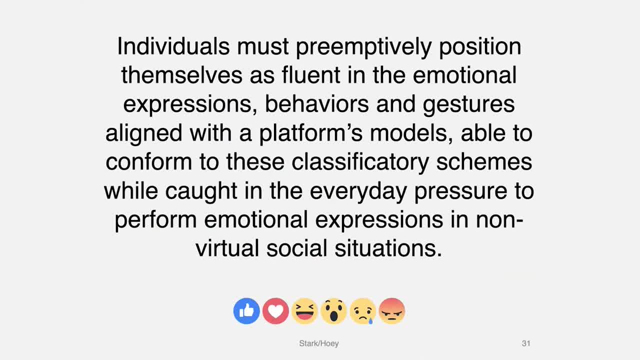 Right, so, um, and so you know, and and the kind of the kind of, the kind of spin-off problem with this, this, this reshaping of our own subjective understanding of emotions around, around motivational models, is, you know who's asking us to do the reshaping, right, You know. and so I think a big concern that 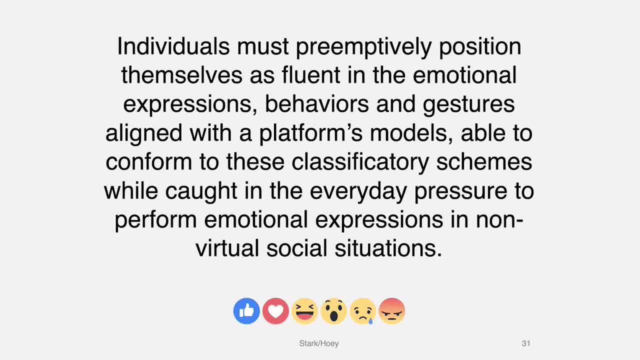 I have with emotion is that individuals will, you know, you know, have to sort of preemptively start positioning themselves, you know, and their emotional expression, as being aligned with the model of platform like Facebook or other platforms, you know, either explicitly or implicitly. 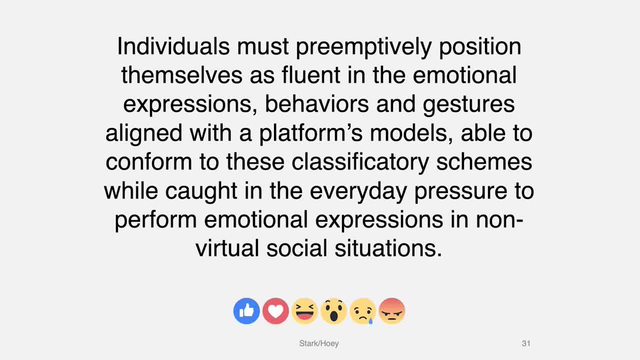 buys into right. You know, we all sort of have to kind of kind of modulate our behavior in different social situations, and so it's people right who are doing the work of you know, understanding how to be legible on social platforms and also in. 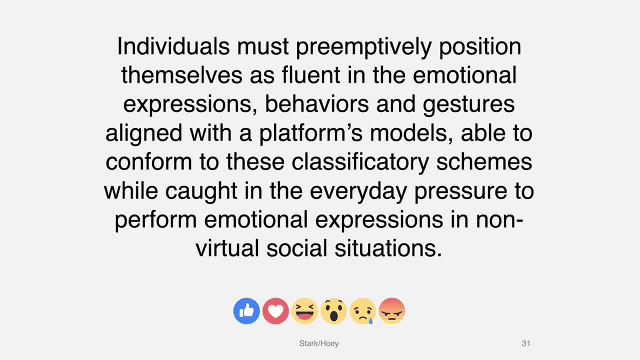 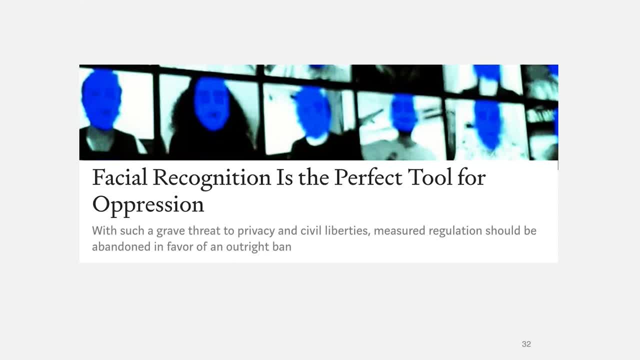 non-social platforms. You know this kind of this kind of modulation you know has big, big big impacts or big, big implications for you know for political discourse, right For conversations about in the civic sphere, about how you know how, how you know our countries and citizens want the world to be run. It's not 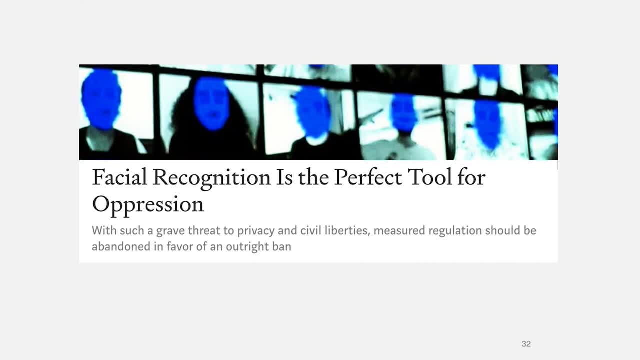 just right that facial recognition is a great tool for oppression, as this piece by Woody Herzog and Ryan Kahlo points out, but it's also that the kind of the kind of way we, as individuals, are shaping our emotional expression and emotional response within social media platforms is 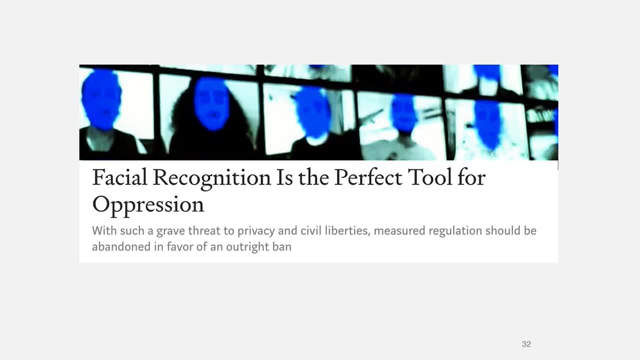 potentially having, you know, having having knock-on effects about civic discourse and and how we communicate with each other, And there's a lot more work to be done, I think, connecting the specific affordances of social media platforms and how they cultivate emotional expression and 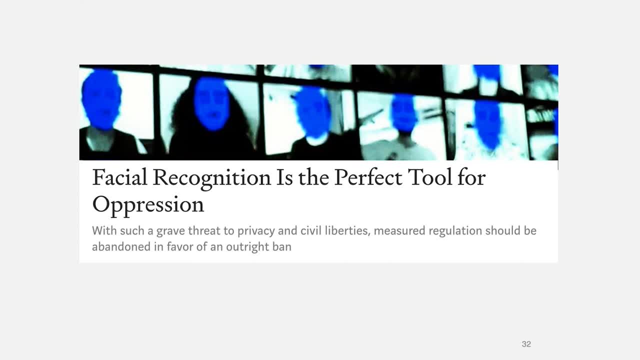 how they collect emotional data. And I think, you know, I think that's a big, big, big big Principle of, of postmodern, or see, of course, you know, like, like çocy, thatي's exist. Perhaps that's what's theяти i' So think about those skills like we, that people like to net palpità. 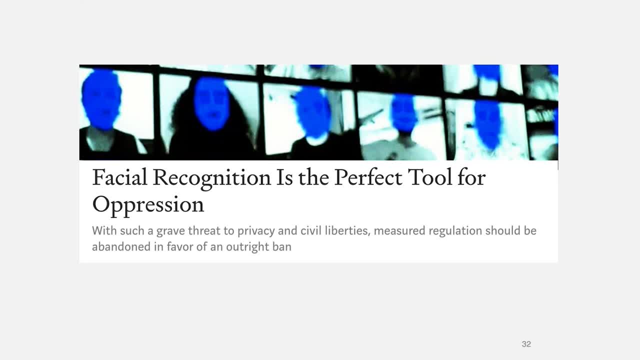 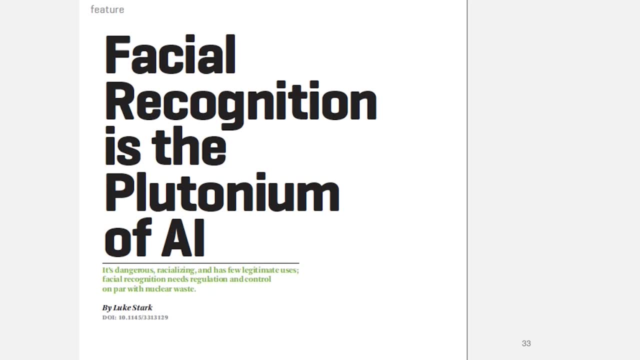 And some of the conversations around polarization, toxicity and the rise of right wing extremism that you know are happening in other other areas of media studies right now, which is why, gifted, I've written that I think that facial recognition especially, and I think, emotional recognition, I'm becoming increasingly convinced. eapู่ emotions five. 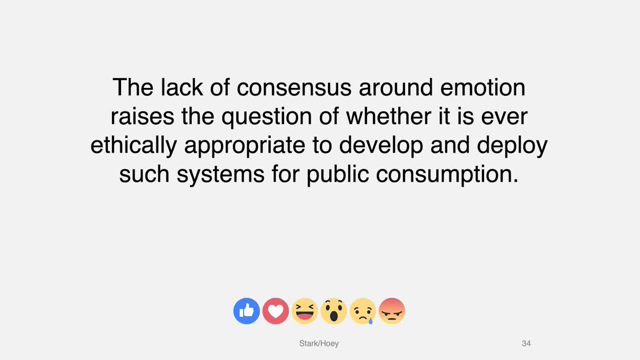 mayor, low. you know, ultimately, finally, you know in in the paper. you know, jesse, and i asked this question right. so we have this total lack of consensus about what emotion is um and uh and what its effects are. right, i mean, they're, they're. it's not that there's like there's no consensus, but there. 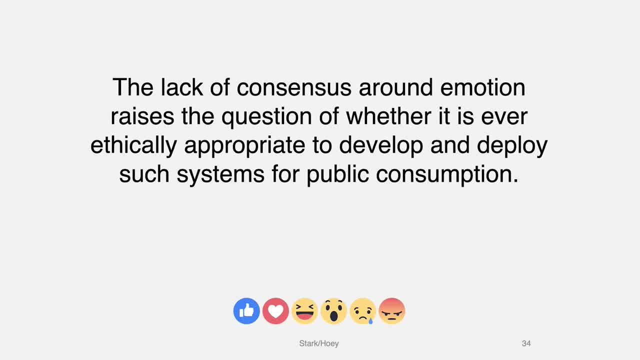 are different camps, um, and, and the problem of parts and the problem of plenty that i talked about at the beginning of this, of this talk, um, you know, really really suggest, right, that effective science itself is highly unsettled and that the, the kind of you know, with quite, quite different, 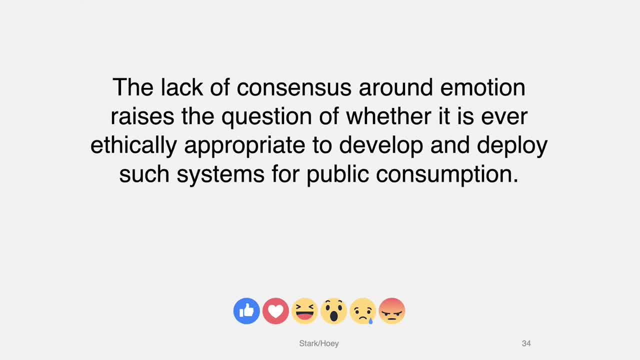 sets of um kind of core conceptual beliefs on different sides of the question. so i think this raises um a bigger question of whether it's ever ethically appropriate to develop and deploy um emotion recognition or emotion analysis systems for public consumption. right, and i'll stress your. 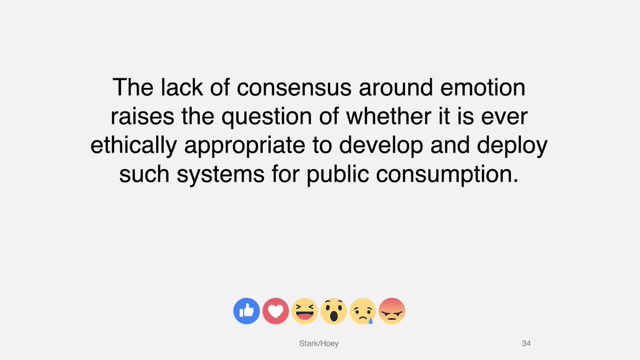 public consumption. right, of course, right. um, there may be, you know, some, some, some relevant or valid reasons to do this work and for research purposes or, in particular, maybe medical or mental health contacts, um, you know, you know, tools for autistic um youth are often brought up as a potential a.